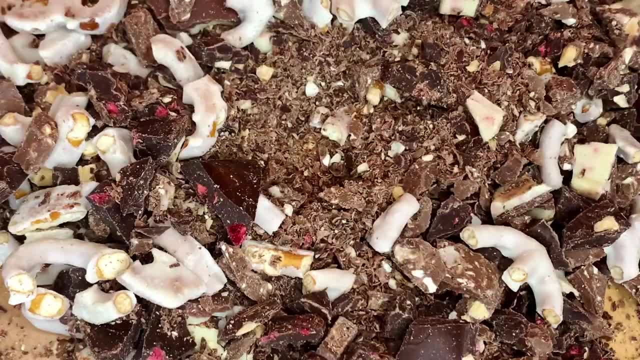 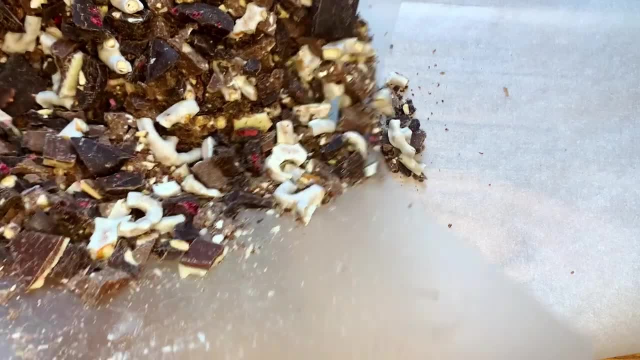 sizes of chocolate pieces all mixed together. I'm going to use a little bit of chocolate to simulate this- and this also represents erosion, the act of removing the broken down pieces from the rock. So the sediment is removed from the rock by erosion and then it's transported by. 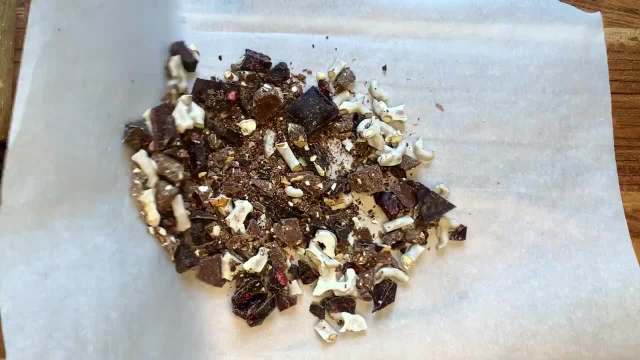 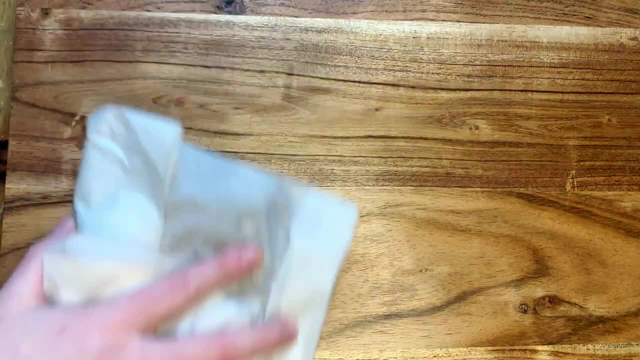 forces like wind or water and deposited somewhere new. Once deposited, sediment eventually gets compacted and cemented together to form a solid rock, a sedimentary rock. This happens through the pressure of other layers of rock and sediment on top of it or burial. I tried to simulate this. 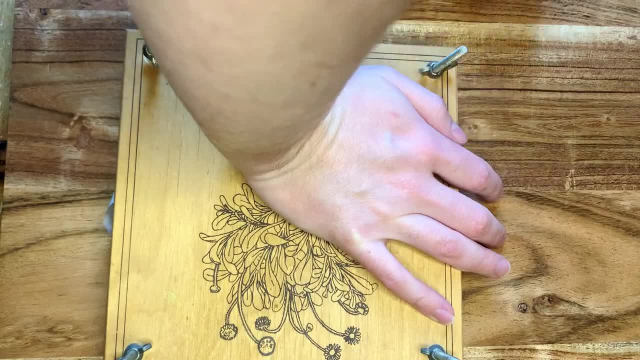 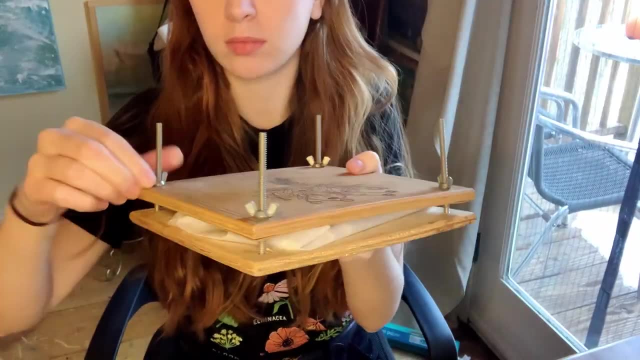 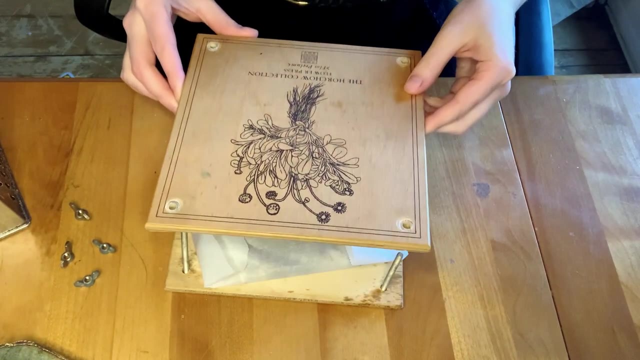 by using a flower press I had lying around, but you could also put the chocolate in a layer of parchment paper and put something heavy on it for a while. I left the flower press for about 45 minutes before my curiosity got the best of me and opened it up. The entire layer wasn't compact. 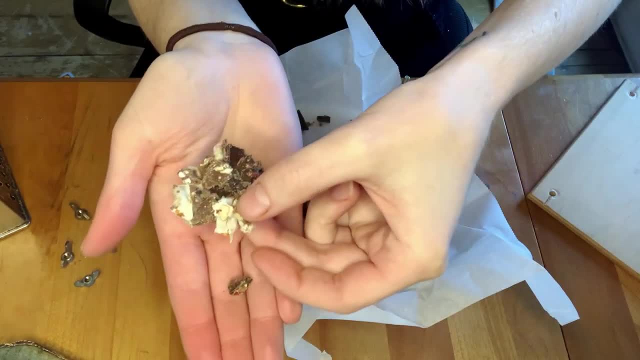 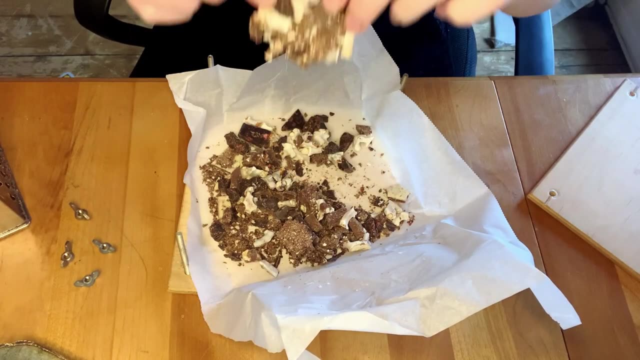 enough to be in one piece, but I did find a few nice pieces that had solidified together into clumps that resembled conglomerate. If I had broken down the chocolate into smaller pieces, I may have gotten a slightly better result. so if you try this, maybe try it this way. 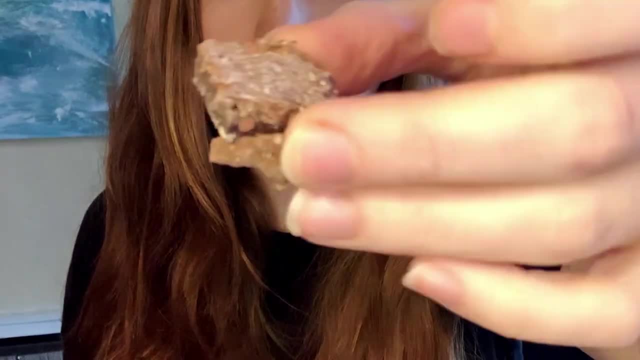 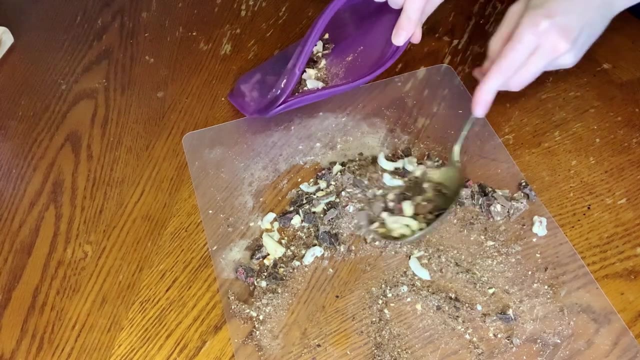 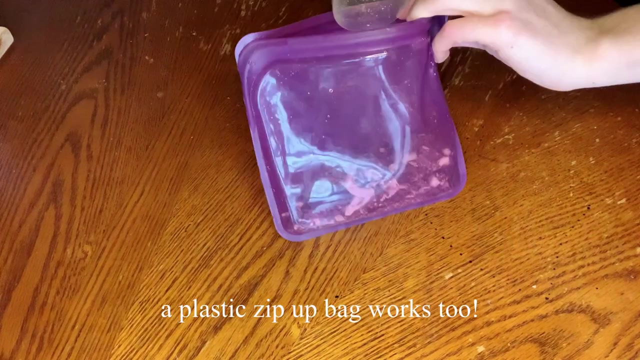 Moving on to the next part of the rock cycle, we have metamorphism. Metamorphism is the process of an existing rock undergoing heat and or pressure that turns it into a different type of rock. I put a bunch of the chocolate pieces into a silicone bag and then I put that bag in a bowl. 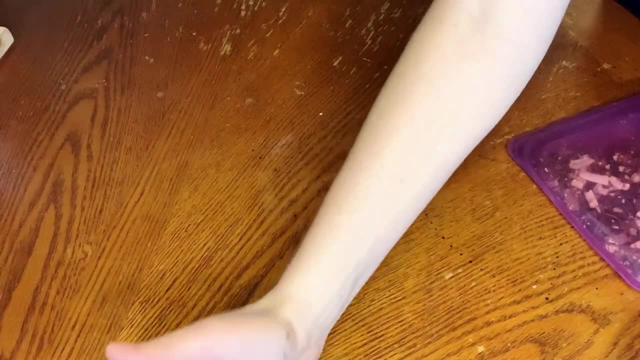 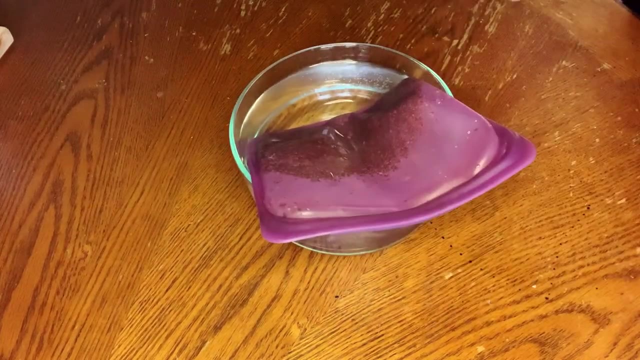 of hot water. These chocolate pieces are supposed to represent an existing solid rock, by the way, not just sediment. So I flipped the bag over after a minute or so in the hot water, and it was already so I squeezed the chocolate around in the bag a little bit to simulate the pressure aspect of 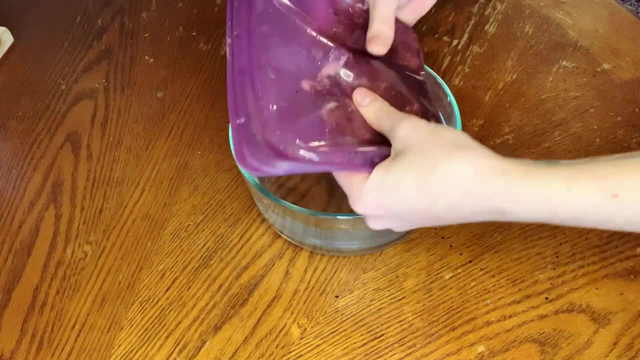 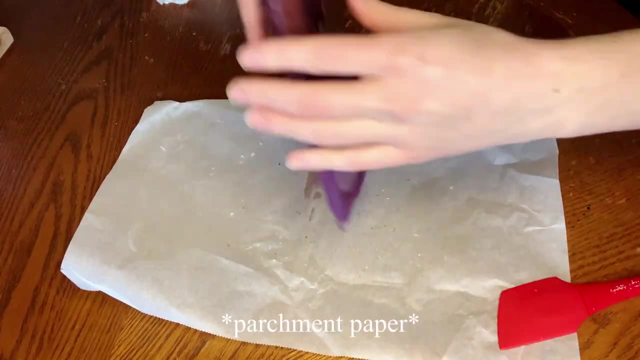 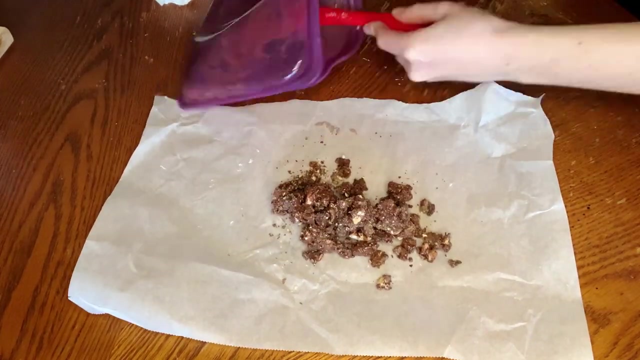 things. Then I dumped it all out on some freezer paper. You can already see a difference from the sedimentary rock I made before this one. I wrapped it up and I squeezed it a little bit more to show how the chocolate was soft enough to morph together as I pressed down. Notice how the chocolate isn't quite melted, just a little softer. so that's a good sign that the chocolate isn't going to melt as quickly as I did before. If you want to see how the chocolate melted, you can click the link in the description box below to see how the chocolate melted, If you want to. 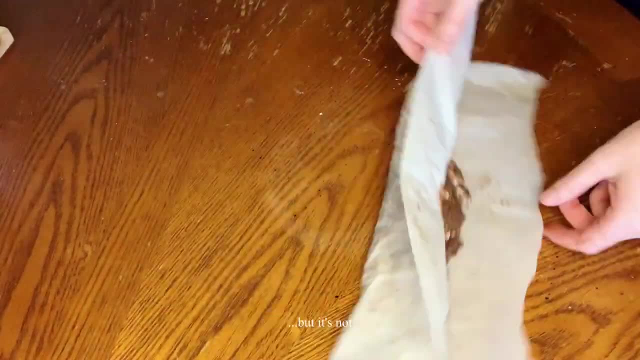 see how the chocolate melted. you can click the link in the description box below to see that I can push the pieces together when I apply pressure. Compare this to the recrystallization of minerals and deformation like foliation and folding in metamorphic rocks. 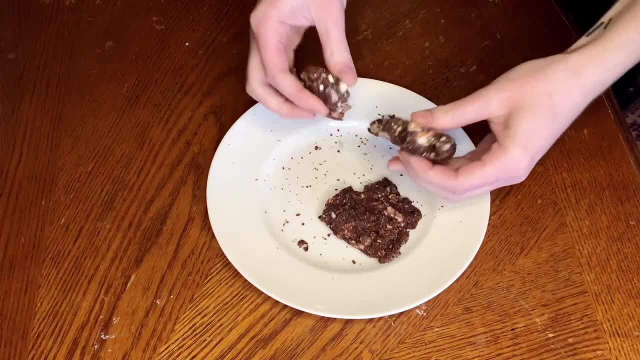 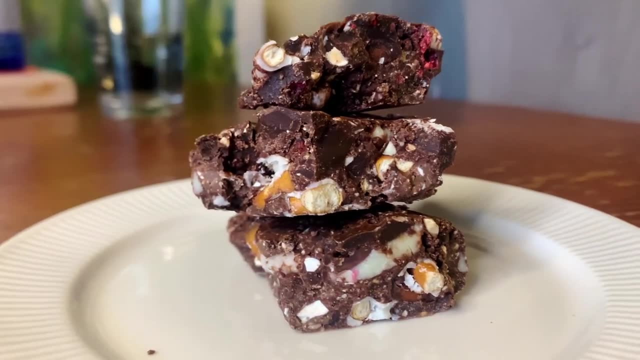 I put that in the freezer for about an hour and when I took it out I broke it open and got a pretty cool result. When you look closely, you can see that the rock is one piece and doesn't fall apart as easily as the sedimentary rock that I made. However, 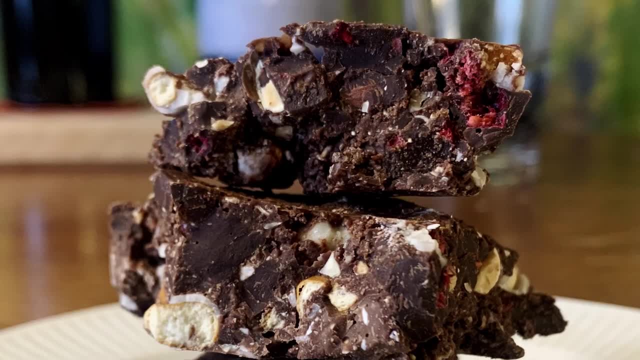 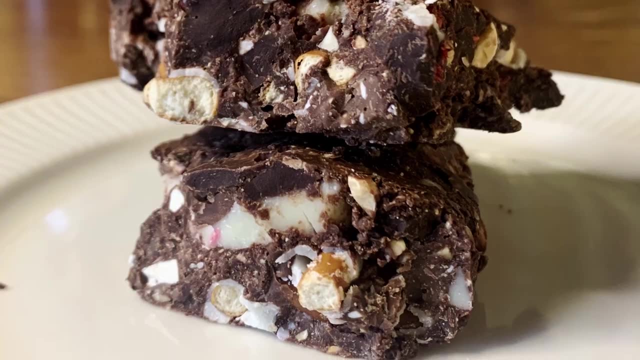 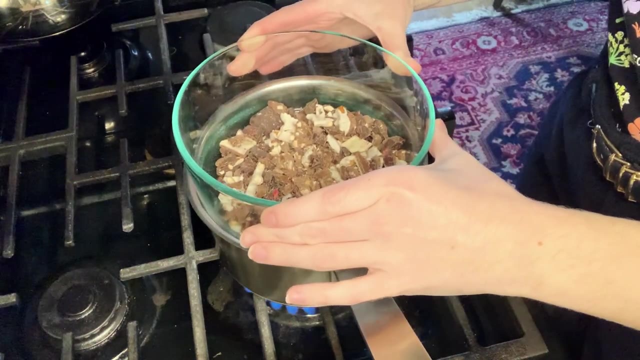 you can still identify different parts of the different chocolates. You can see the white chocolate still surrounding pretzel pieces, chunks of dark chocolate and white chocolate surrounded by morphed milk chocolate. Let's see how different it looks when we melt the chocolate instead. Next up in the rock cycle, we are going to show how any type of existing rock can become. 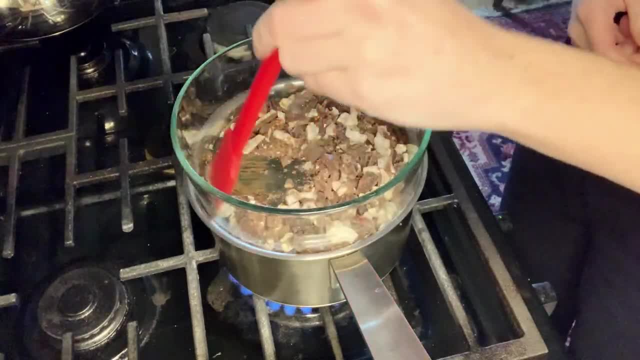 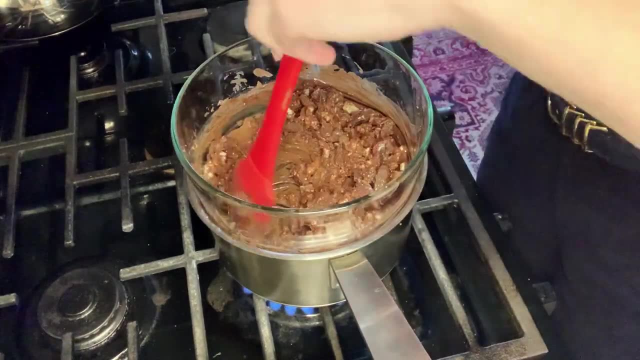 magma and then igneous rock. I put a pot of water on medium to low heat and I put a Pyrex bowl with chocolate pieces inside. This is to simulate the process of turning rock- any type of rock- into magma. Rock gets pushed deep underground and through different processes, 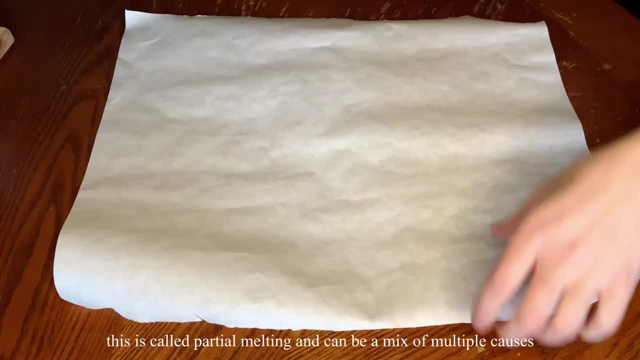 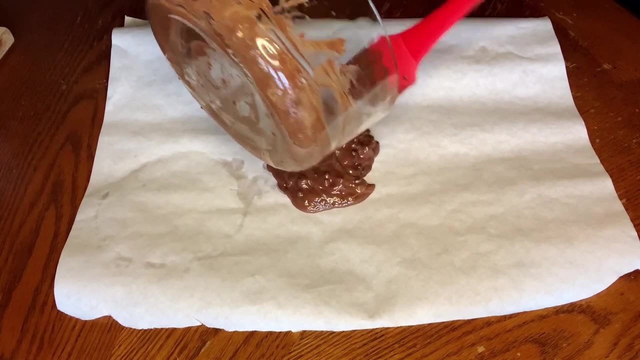 melts into molten rock. This can occur because of heat decompression or addition of volatiles like water, which lower the melting point of minerals in the rocks. The minerals within rocks have different melting points, so some melt at certain conditions, while 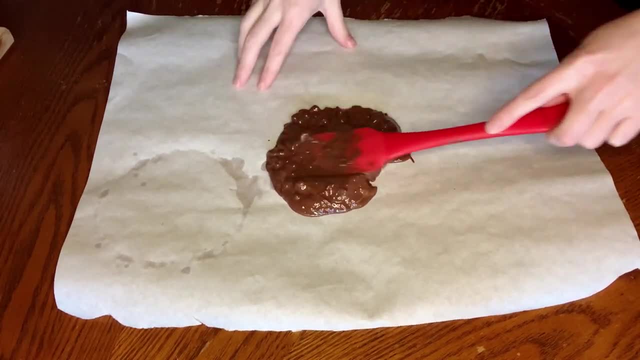 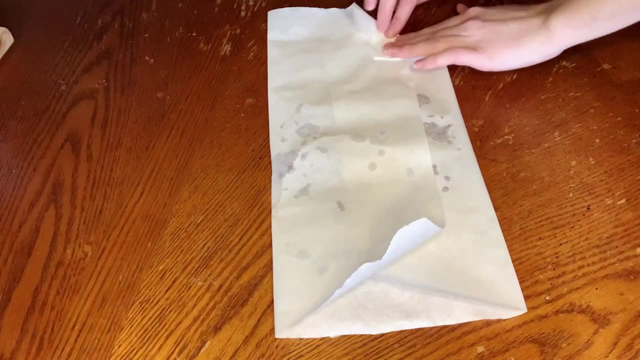 others are a little bit tougher. You can compare this to the almonds and pretzels: that remain solid while the rest of the chocolate softens. I poured the mixture onto some parchment paper and I put that in the freezer for about an hour so it could solidify. This represents the crystallization of 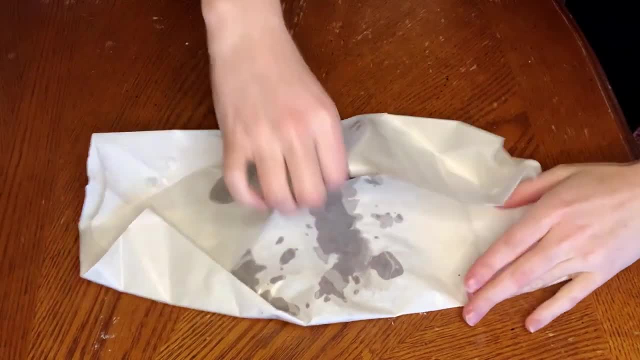 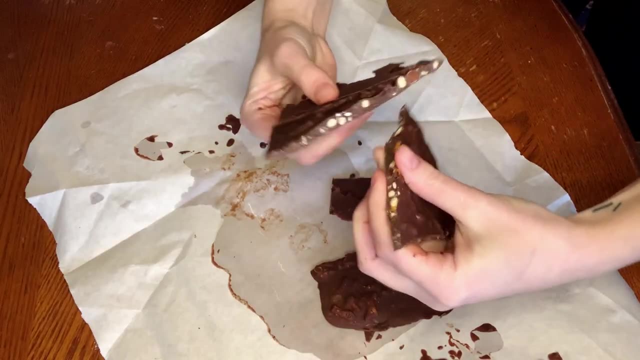 magma in the earth's crust as it cools. It could also represent the cooling of lava at the surface. When it was solid, I took it out of the freezer and broke it apart to see the results. You can see some similarities here to the metamorphic rock, but the chocolate is mostly. 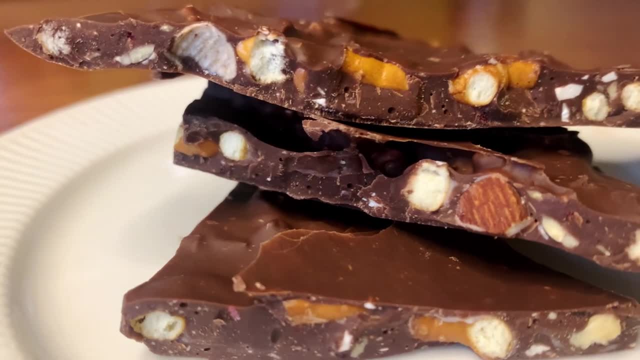 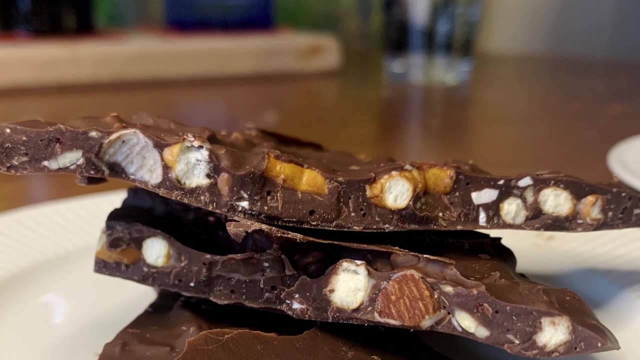 the same color here. The main visible aspects of this are the chocolate and the solid non-chocolate pieces like pretzels and almonds. There's also no longer white chocolate covering the pretzel pieces and you can't see separate pieces of dark chocolate and white chocolate. It's all kind of 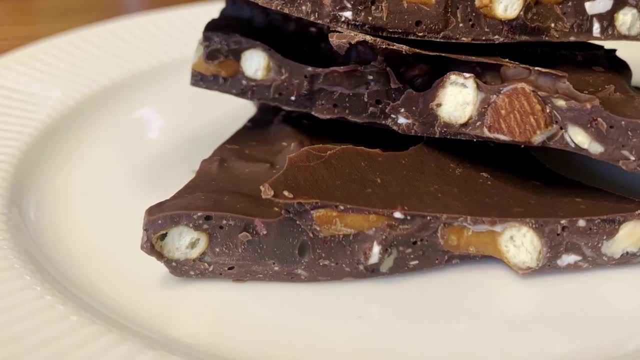 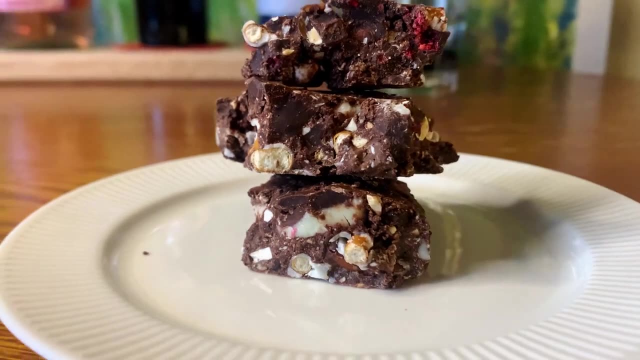 just one big chunk of chocolate. now There are even some vesicles in there which are very fitting for an igneous rock. Here's another clip of the metamorphic rock. At this point in the rock cycle, anything can happen. The igneous rock could be turned.